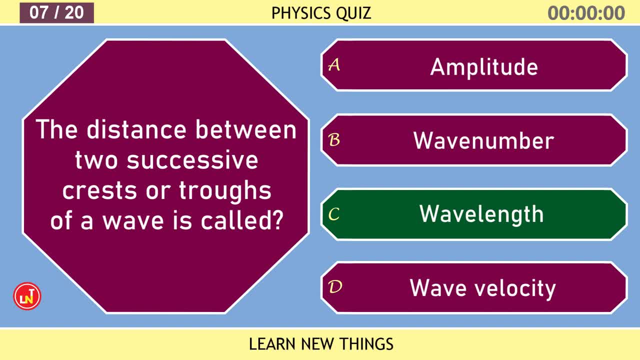 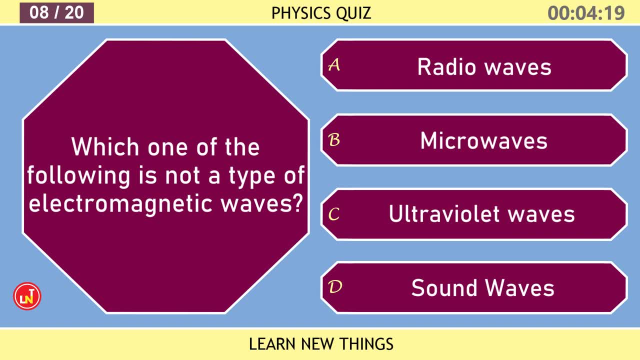 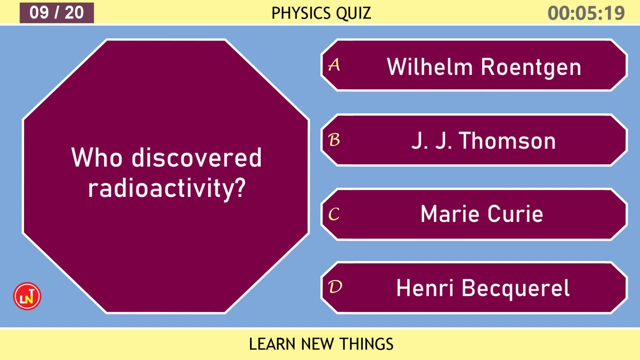 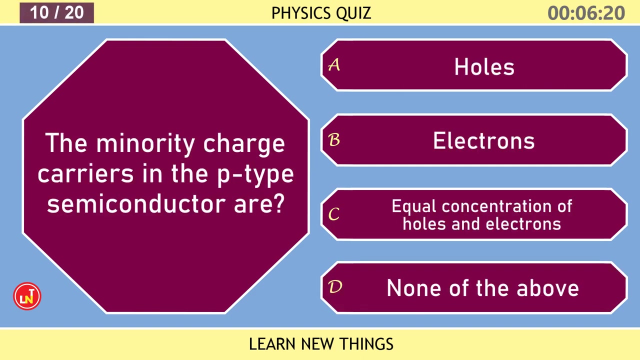 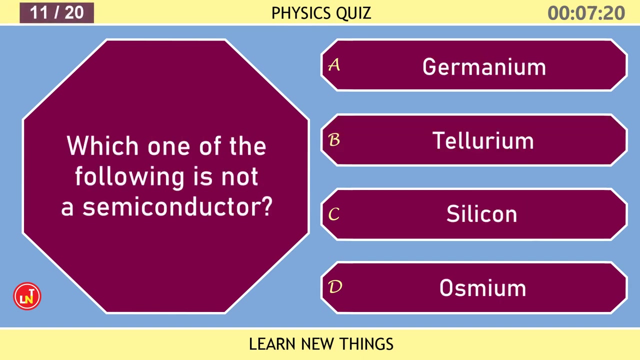 Wavelength? Which one of the following is not a type of electromagnetic waves: Sound waves? Who discovered radioactivity? Henry Becquerel. The minority charge carriers in the p-type semiconductor are P-type, P-type Electrons. Which one of the following is not a semiconductor? 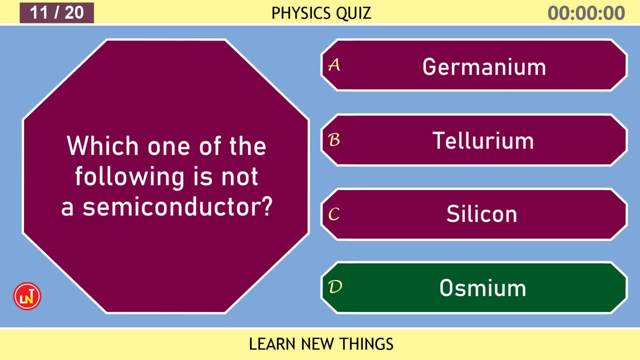 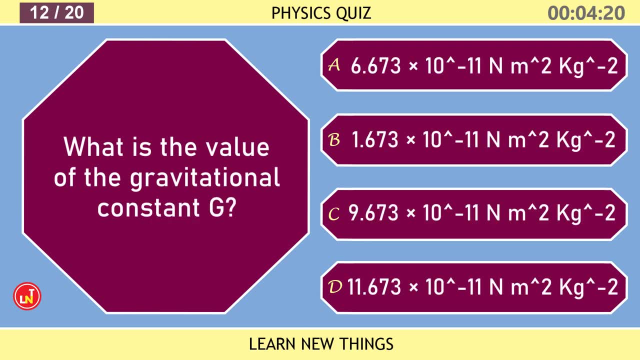 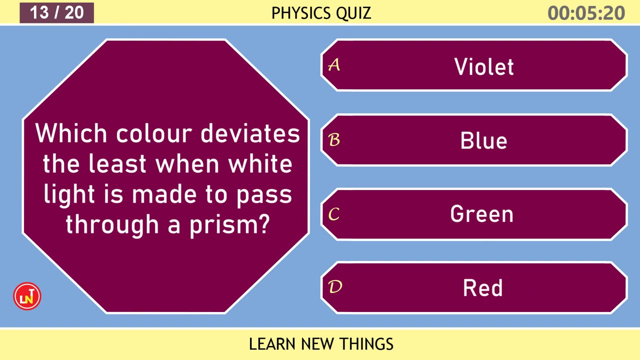 Osmium. What is the value of the gravitational constant G System of the solar plexus? Answer is Option A. Which color deviates the least when white light is made to pass through a prism Red. The 4th state of matter is Dash. 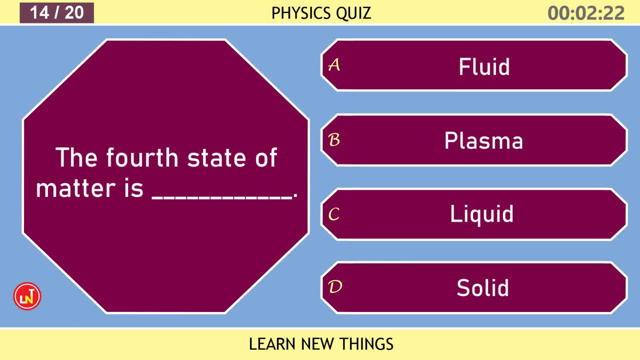 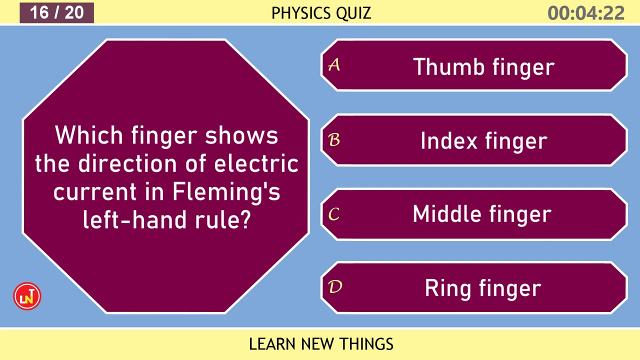 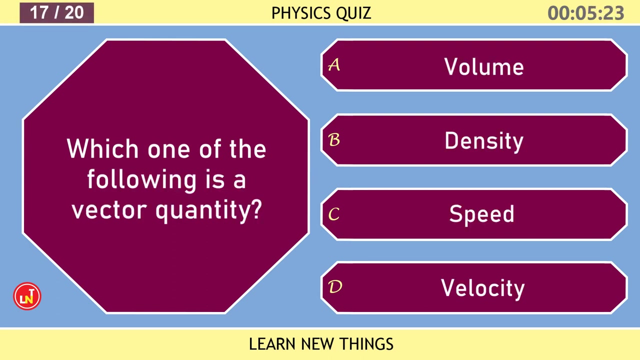 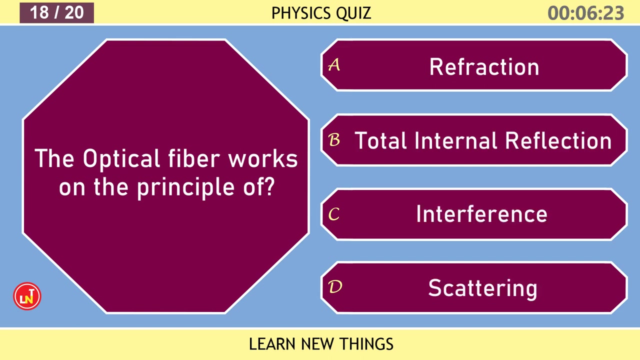 Plasma? What is the focal length of a plane mirror? Infinity? Which finger shows the direction of electric current? in Fleming's left hand rule, Middle finger, Which one of the following is a vector quantity: Velocity? The optical fiber works on the principle of Total Internal Reflection.